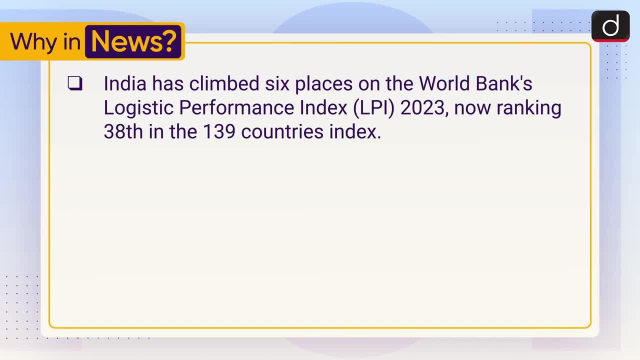 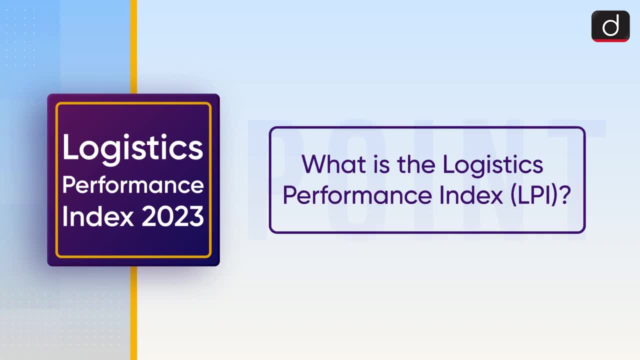 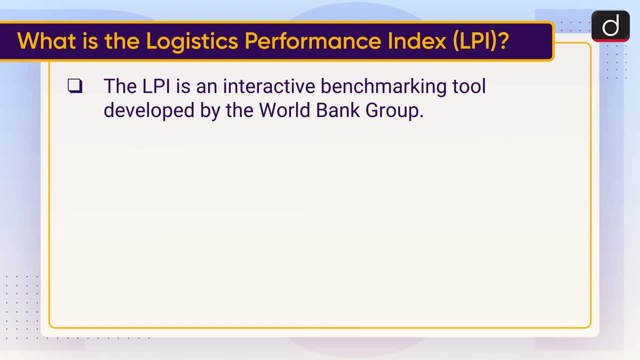 now ranking 38th in the 139 countries index. Now let's discuss what is the Logistics Performance Index, or LPI? The LPI is an interactive benchmarking tool developed by the World Bank Group. It helps countries identify the challenges and opportunities they face in their performance. 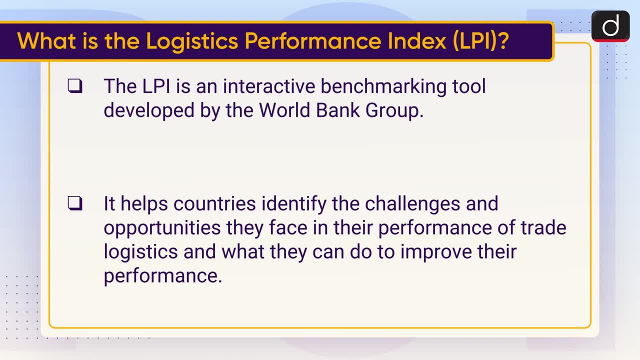 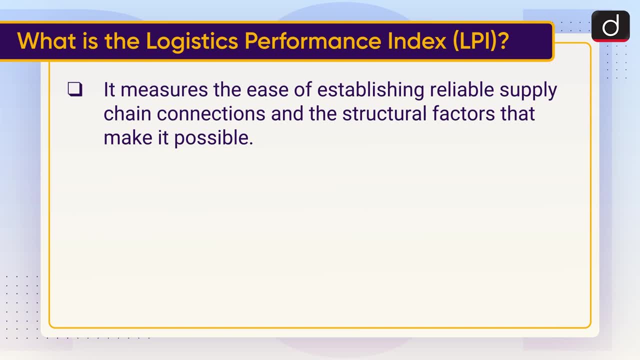 of trade logistics and what they can do to improve their performance. It measures the ease of establishing reliable supply chain connections and the structural factors that make it possible. The LPI was reported by the World Bank every two years from 2010 to 2018, with a break. 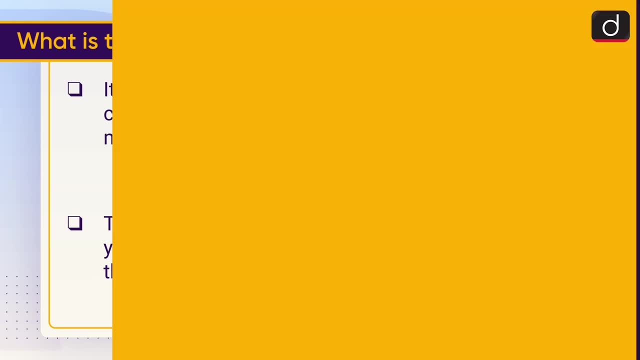 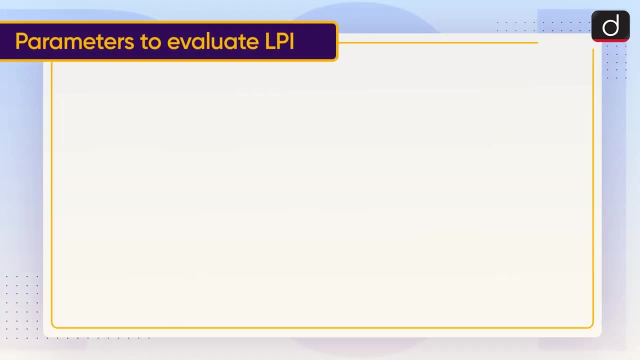 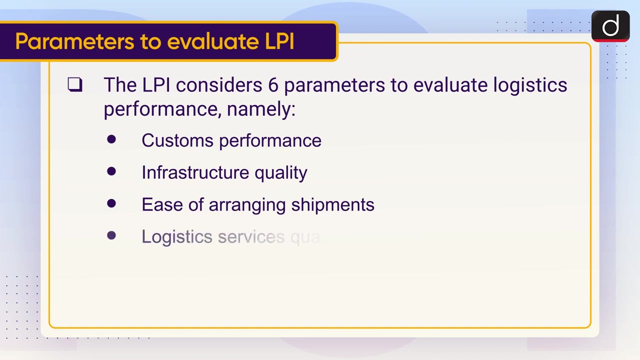 in 2020 due to the covid 19 pandemic. now moving on to the parameters to evaluate lpi. the lpi, that is, logistics performance index, considers six parameters to evaluate logistics performance, namely customs performance, infrastructure quality, ease of arranging shipments, logistics services quality, consignment, tracking and tracing and timeliness of shipments. 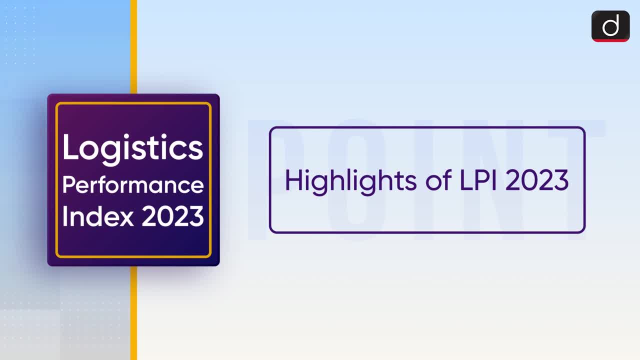 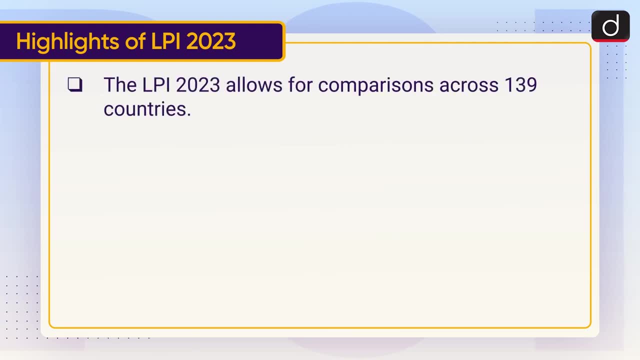 now let's have a look at the highlights of lpi 2023. the lpi 2023 allows for comparisons across 139 countries. the lpi 2023, for the first time, measures the speed of trade with indicators derived from big data sets tracking shipments. 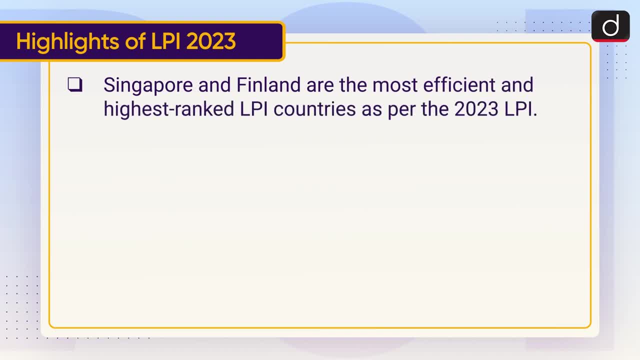 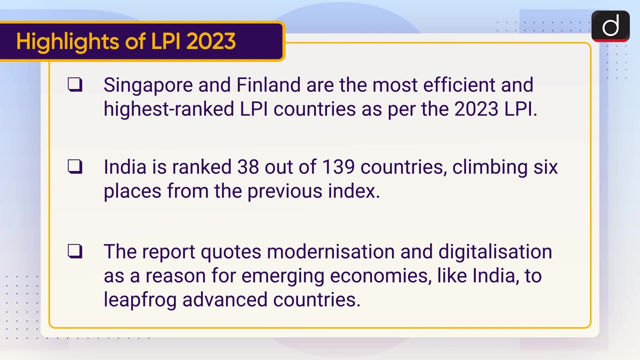 singapore and finland are the most efficient and highest ranked lpi countries. as per the 2023 lpi, india is ranked 38 out of 139 countries, climbing six places from the previous index. the report quotes modernization and digitalization as a reason for emerging. 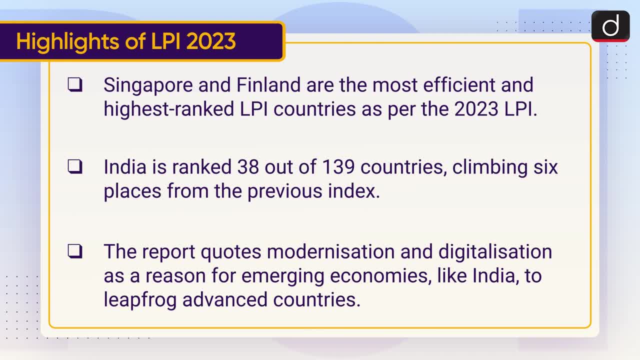 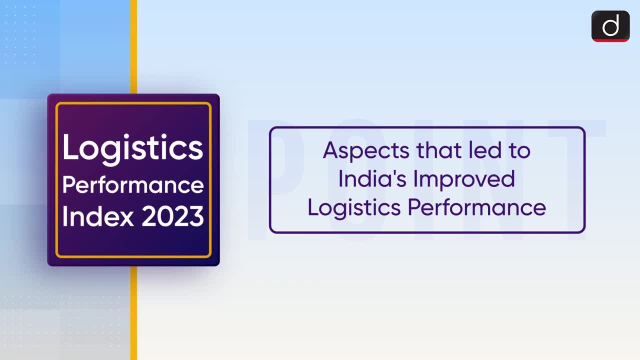 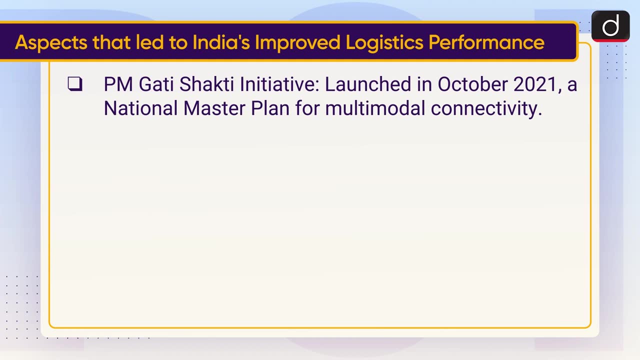 economies like india to leapfrog advanced countries. now let's understand about the aspects that led to india's improved logistics performance: pm gati shakti initiative, launched in october 2021. a national master plan for multimodal connectivity- national logistics policy or nlp, launched in 2022 to ensure quick last mile delivery and desired 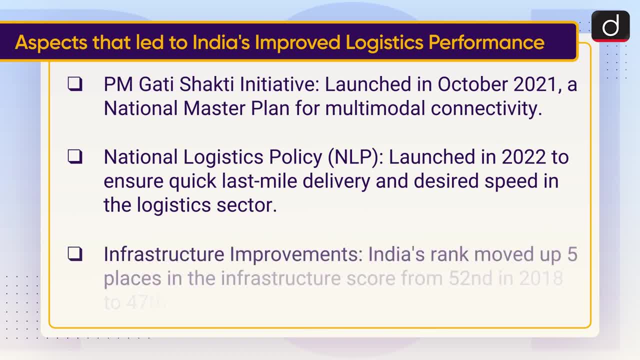 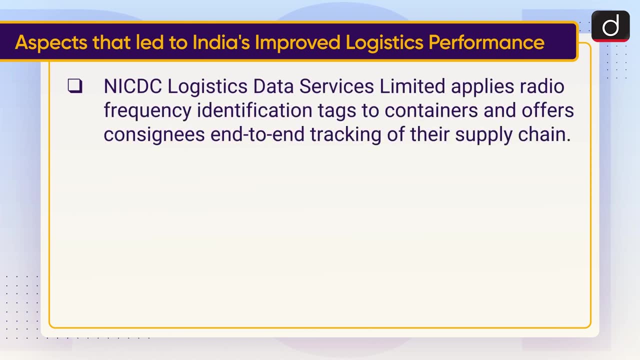 speed in the logistics sector infrastructure improvements. india's rank moved up five places in the infrastructure score from 52nd in 2018 to 52nd in 2021.. in 2023, nicdc logistics data services limited applies radio frequency identification tags to. 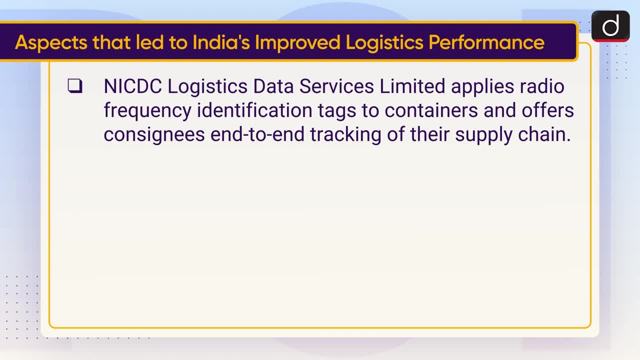 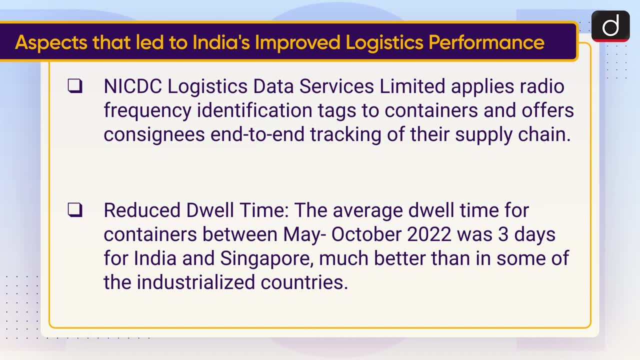 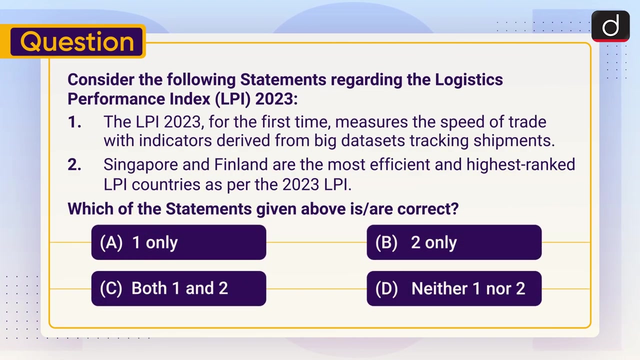 containers and offers consignees end-to-end tracking of their supply chain and reduced dwell time. the average dwell time for containers between may to october 2022 was three days for india and singapore- much better than in some of the industrialized countries. now it's time for the practice question. consider the following statements regarding the logistics. 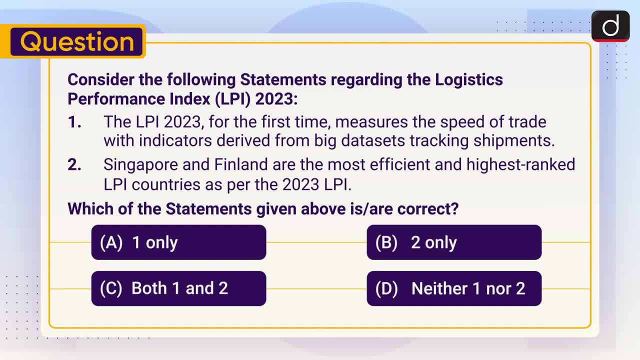 performance index or lpi 2023. one: the lpi 2023, for the first time, measures the speed of trade with indicators derived from big data sets tracking shipments. two: singapore and finland are the most efficient and highest ranked lpi countries as per the 2023 lpi. which of the statements given above? 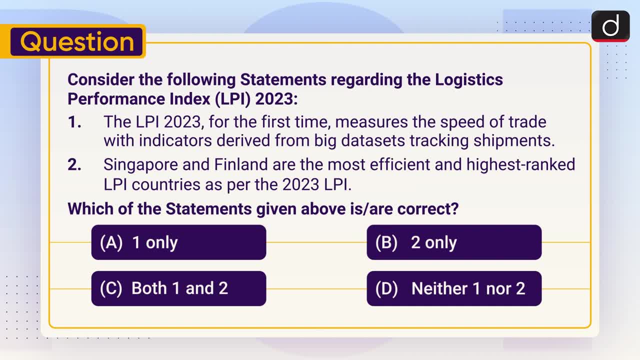 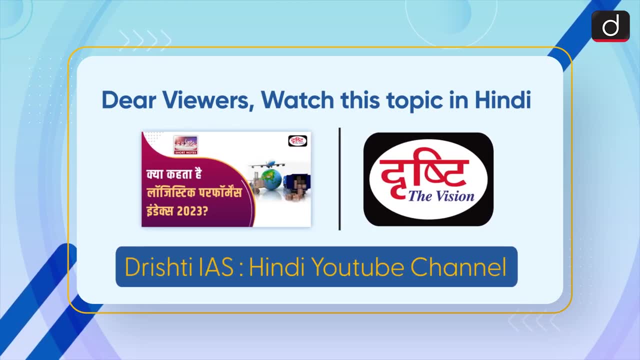 is or are correct one only two, only both, one and two or neither one nor two? send the answer of this question in the comment section. stay tuned for the next episode. thanks for watching. have a great day, dear viewers. watch this topic in hindi on our drishti is in the youtube channel.